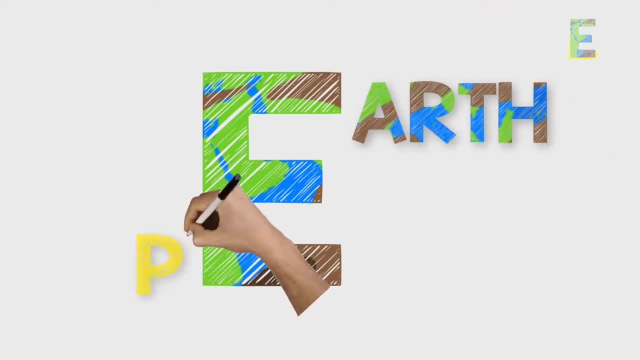 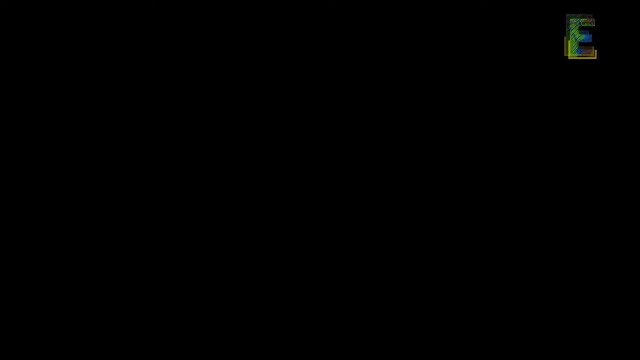 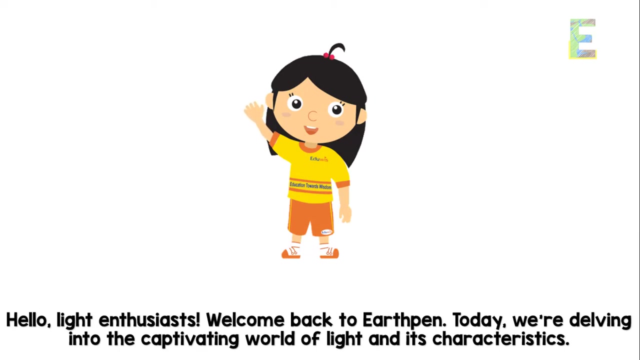 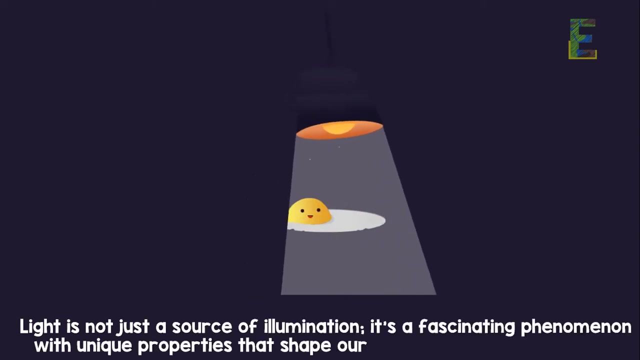 Hello, light enthusiasts, Welcome back to EarthPen. Today we're delving into the captivating world of light and its characteristics. Light is not just a source of illumination. it's a fascinating phenomenon with unique properties that shape our understanding of the world. 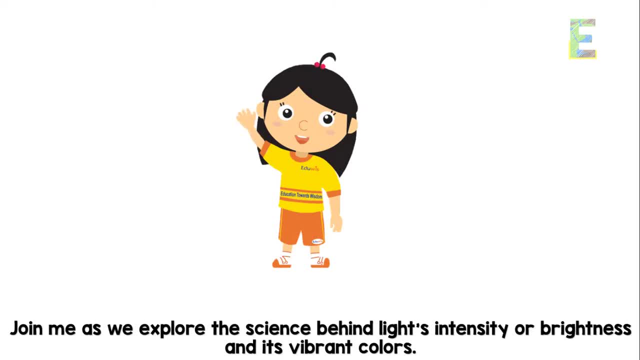 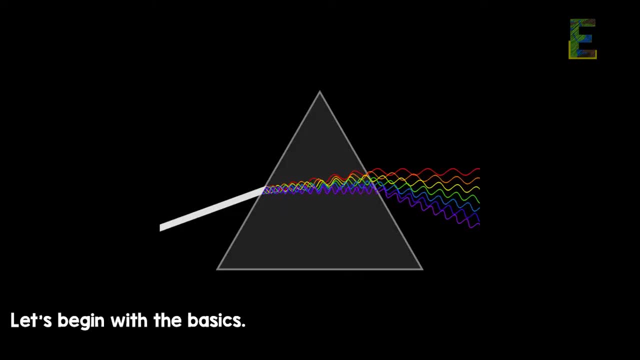 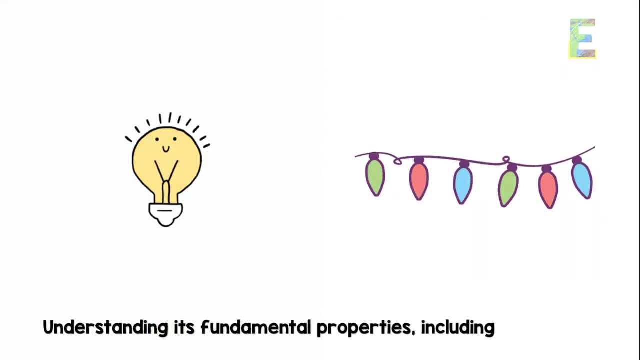 Join me as we explore the science behind light's intensity or brightness and its vibrant colors. Introduction to light characteristics. let's begin with the basics. Light is a form of electromagnetic radiation that travels in waves. Understanding its fundamental properties, including intensity or brightness in color, helps us comprehend the nature of. 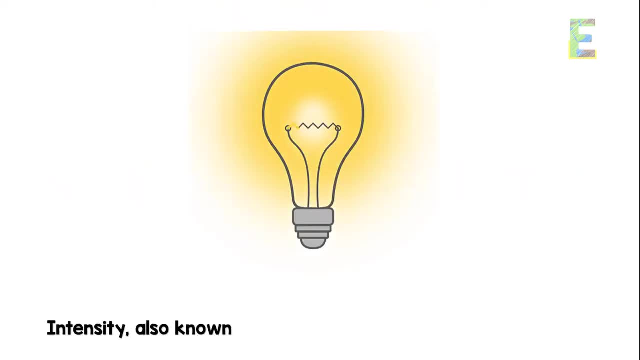 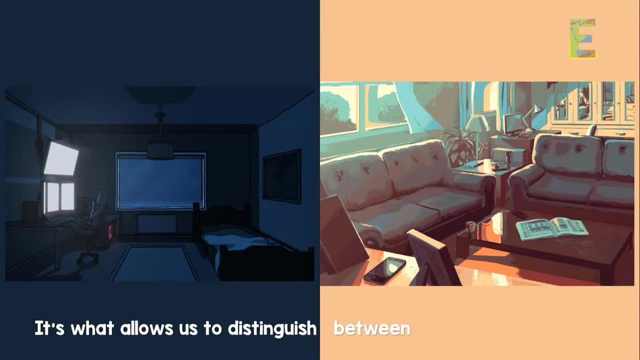 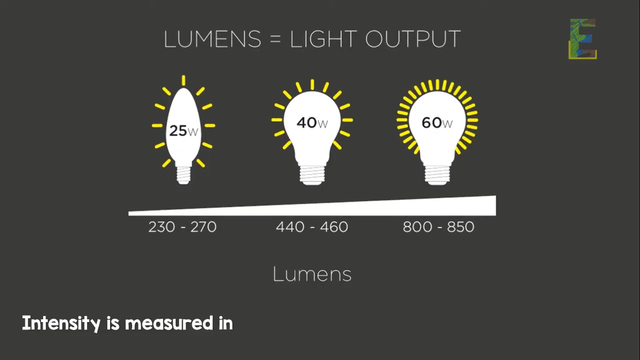 light Intensity or brightness intensity, also known as brightness Light, refers to the amount of light energy in a beam. It's what allows us to distinguish between a dimly lit room and a brilliantly sunlit day. Measuring intensity: intensity- 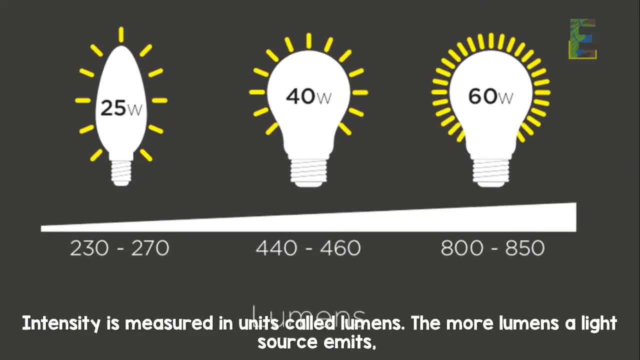 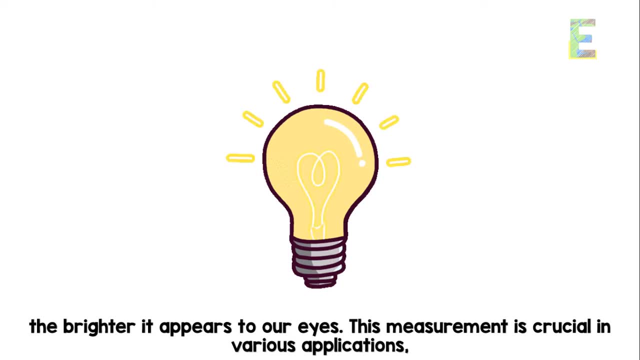 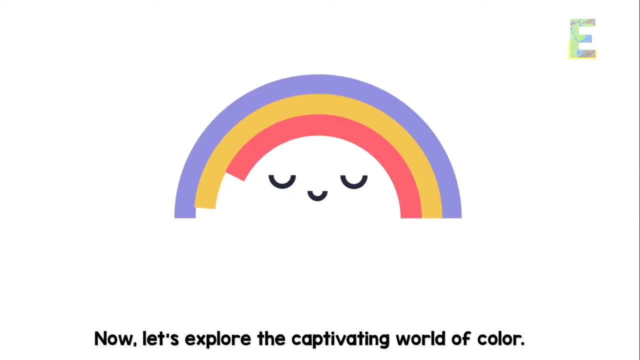 is measured in units called lumens. The more lumens a light source emits, the brighter it appears to our eyes. This measurement is crucial in various applications, from photography to designing efficient lighting systems. Color- now let's explore the captivating world of color. 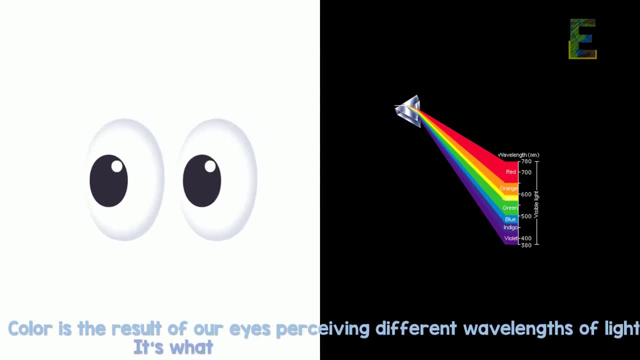 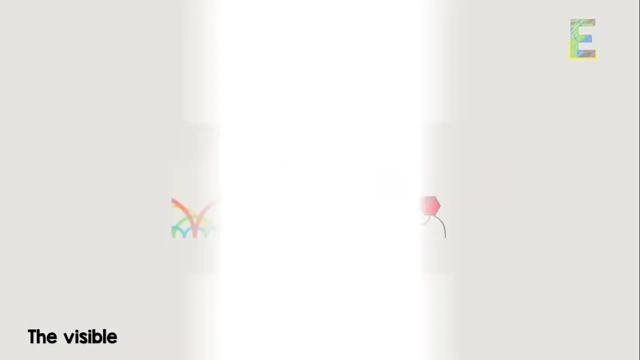 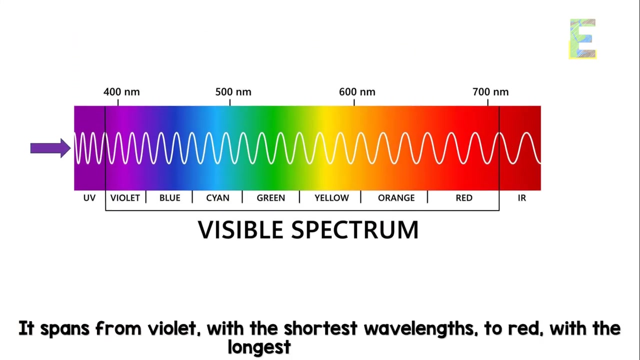 Color is the result of our eyes perceiving different wavelengths of light. It's what gives the world its visual richness: The visible spectrum. the visible spectrum is the range of colors our eyes can perceive. It spans from violet with the shortest wavelengths. 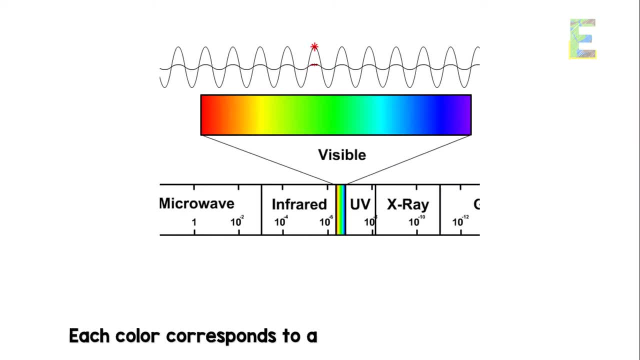 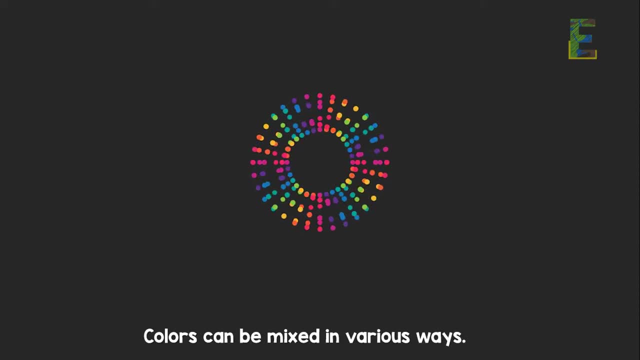 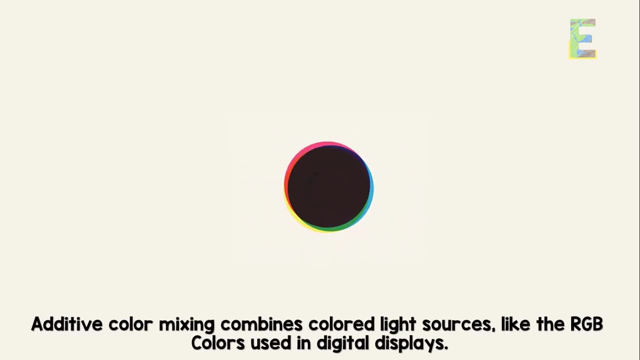 to red with the longest wavelengths. Each color corresponds to a specific wavelength of light. Color mixing colors can be mixed in various ways. Additive color mixing combines colored light sources like the RGB colors used in digital displays. Subtractive color mixing occurs when pigments or filters are combined. 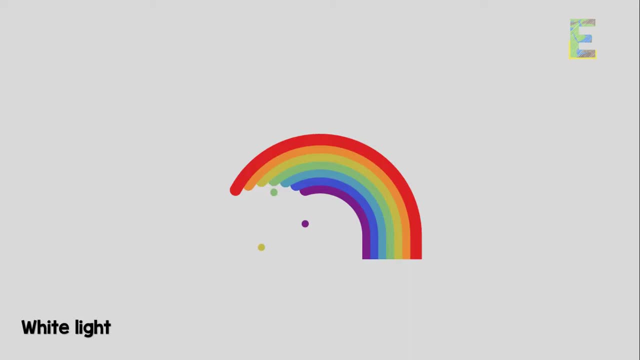 such as in painting or printing White light. white light is a fascinating aspect of color. It's not a single color, but a mixture of all colors in the visible spectrum. When white light passes through a prism, it disperses into a spectrum of colors revealing.